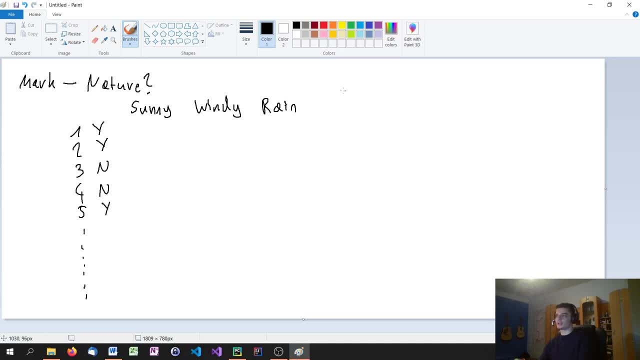 or not, if it was raining or not, and also if he was alone or not. So, uh, one of the criteria is maybe is he going alone into nature or is someone going with him? And we have a bunch of different. 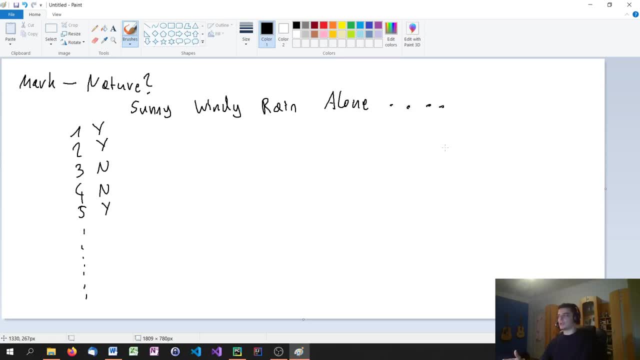 uh, parameters that we can look at, and then we have the decisions. For example, he went out into nature. it was sunny, it was not windy, it was not rainy, but he was alone. Oh, actually, this is a yes. then He was alone. Uh, then he also went out when it was windy, not raining, and he wasn't. 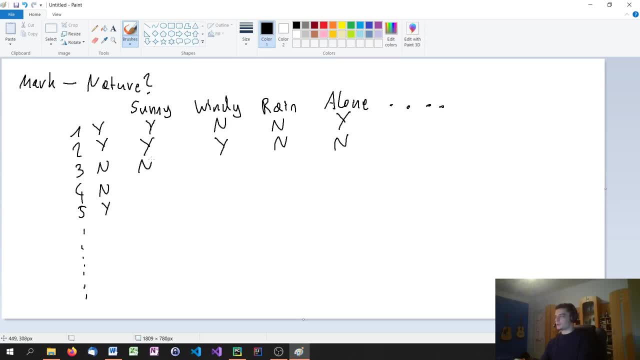 alone. Then there was a way, uh, a day which was not sunny, very windy, very rainy, and he was also alone. So we didn't go, And what we have is we have this data set of events of: did he go out or 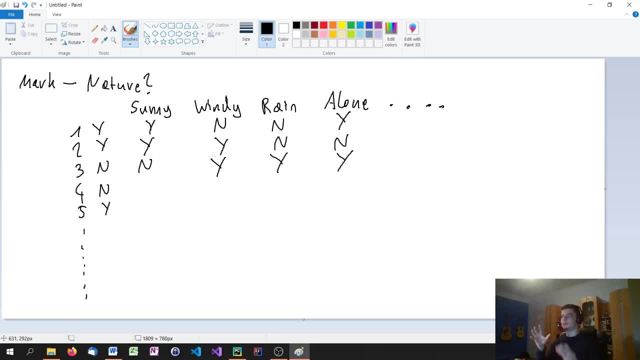 not. And what we try to do now is we try to build a model, a decision tree model that predicts the right uh answers. So what we do is we give that decision tree uh the data. if the day is sunny, 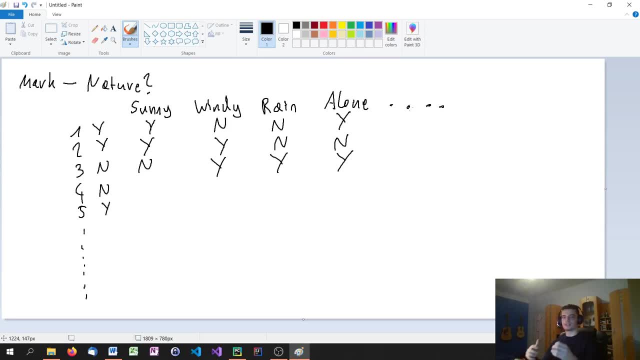 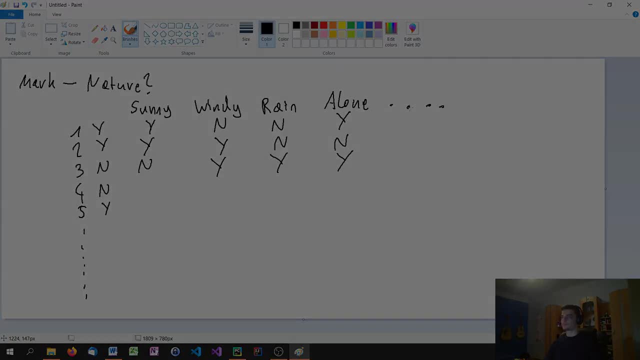 if it's windy, rainy if he's alone, and other parameters in the decision tree. in the end, uh ends up with a classification which is yes or no, Is he going out Or not? So let's look at what a decision tree like this would look like. Um, basically, would. 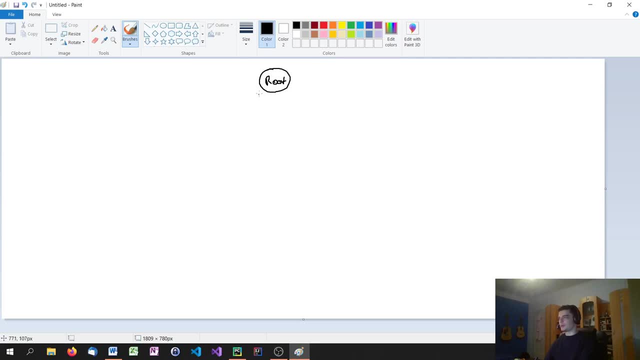 have a route. If the decision tree is already trained, we would have a route that goes off into two branches, And these branches could be: uh, it's sunny or not sunny, And then we have another point here. The next question is: uh, does it rain? question mark. And we could say: 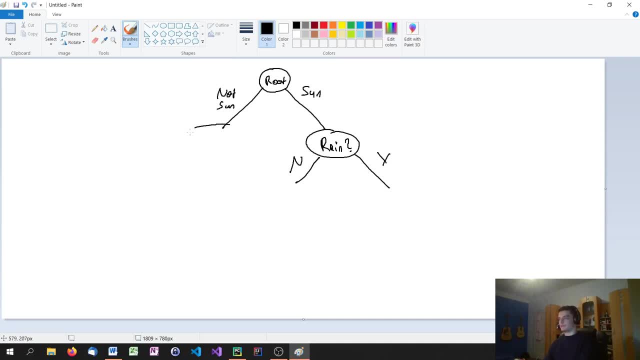 yes, it rains or no, it doesn't rain. And if it's not sunny also, we can ask: does it rain? We can get a no and a yes, And then we could have the question of: is it windy? Then we could again get yes, No. 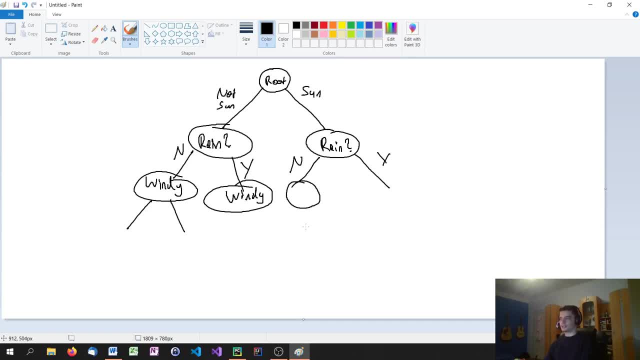 we could also have windy in every other branch. or maybe it's obvious to the decision tree that if it rains, I'm not going anyway, or he's not going anyway, So I don't even have to check for anything else. We have a decision tree that we just have to answer. a couple of questions. 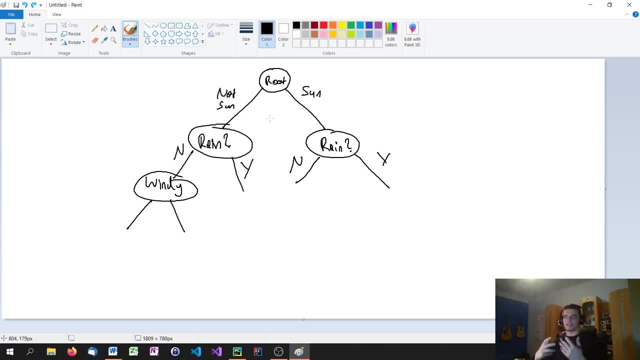 So if yes and no questions, uh, or actually it doesn't have to be yes or no. We could also answer: uh, sunny, windy, cloudy, whatever, If we have multiple options, not only binary options, um, we just answer some questions And in the end we end up with an answer that is either yes, 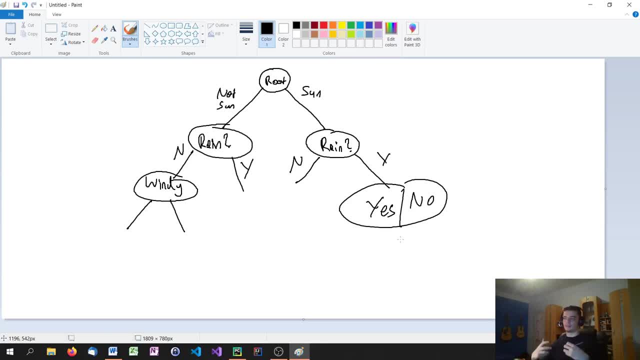 or no, or it also could be, in the example of the breast cancer data set, malignant or benign, Uh, or actually we could also have three different classes, So it doesn't have to be limited to just two Uh. but basically this is, uh, how the decision tree works once it's trained. 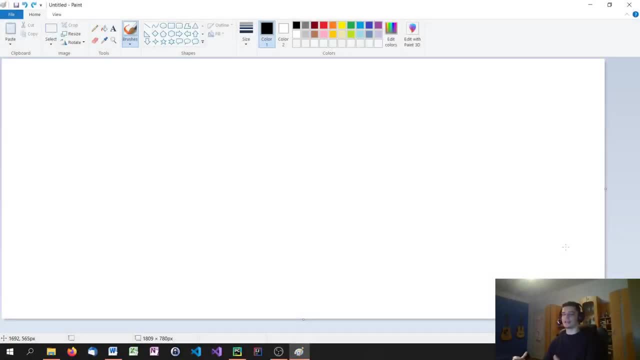 So the question remains: how do we train that model, or how is that model being trained in Python, for example? Now, what we do in the beginning is we define a root node and this root node asks one question. So it is a random question. We choose a random feature, for example: 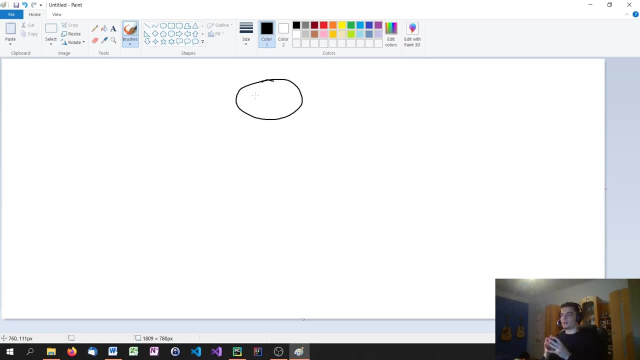 sunny, rainy, or is he alone? And then we split up the possibilities into different branches. So, for example, the first question, is it sunny or not? And then I can get either a yes or a no. So yes or no, Of course, if I have. 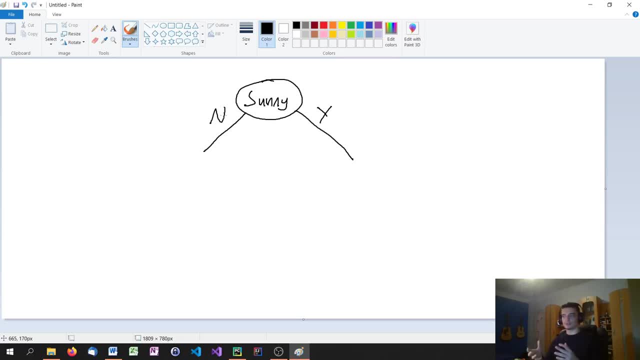 a column or a feature that has multiple options, not only two. uh, I can also, uh, have three or four or five branches, or 10,000 branches. So I could say: sunny yes, sunny no, or I could 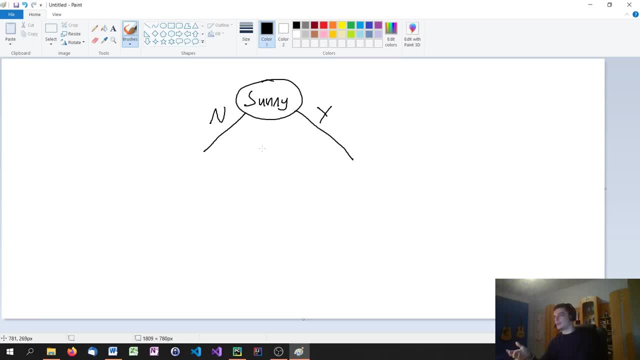 generally ask for the weather, and then I could say sunny, rainy or whatever, And I can have like five possibilities here. Uh, then what I can do is I can say, uh, is it sunny or not? And then I can do is I have the data set, or we have the data set from the beginning, where we have all these. 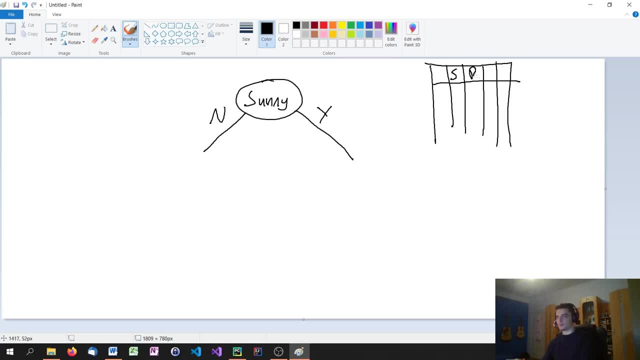 columns, basically, And we have the column- sunny and rainy and alone- And then we had a conclusion if he's going or not. And what we're doing now is we're splitting up the data set. So I have a bunch of yeses here in the sunny column and a bunch of nos, And what I now do is I get all the 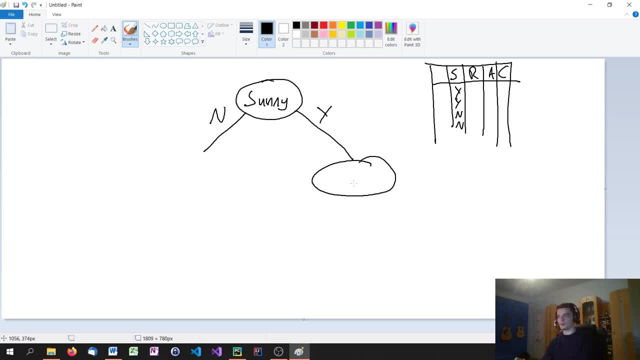 yeses on the right side. So I get all the rows that have a yes on sunny on the right side and all the nos on the left side. Uh, and what I do now is I check for how many of the right side, how many of the data rows here on the right end up being a yes or a no. Finally, in the final, 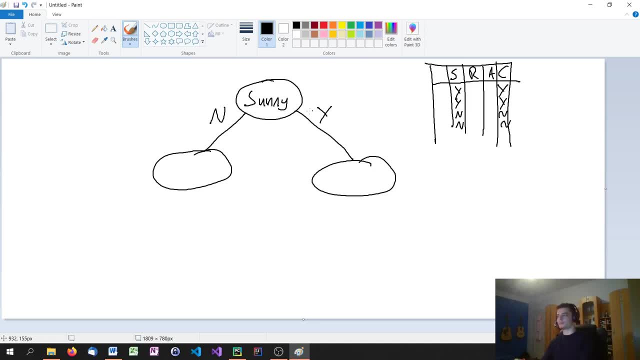 answer is he going out or not, And then I keep track of that number, For example, uh in in this data set. it might be the case that he always goes out when it's sunny. In this case, I would get. 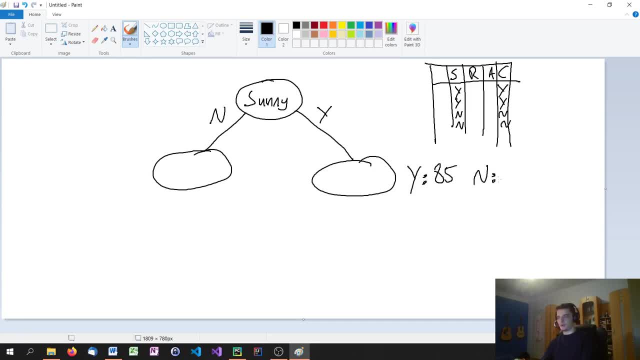 for example- I don't know- 85 yeses and zero nos, And if this is the case, what I can do is I can already say if it's sunny, the decision tree ends here And I give you a final yes prediction, because I don't have to check if it's rainy or if 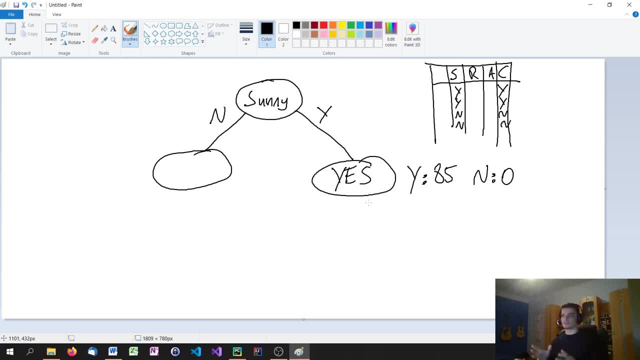 he's going alone. If, if it's sunny, he always goes. So this is at least what the data set tells us. Um, whereas if it's not sunny, I have, uh, for example, 30 yeses and 55 nos. Uh, actually it's. 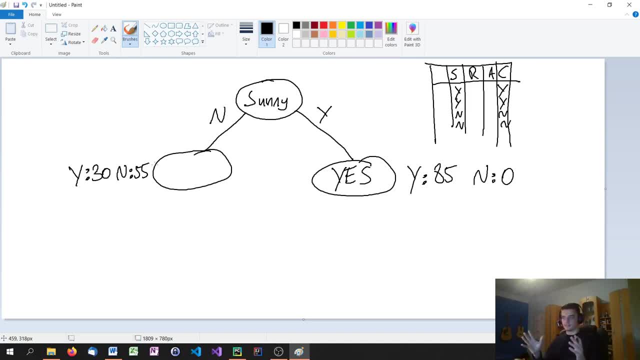 it's a coincidence that they both add up To 85.. It doesn't have to be the same number. We could also have, uh, 200 examples here and 85 here, It doesn't matter, But in this case we have 85, 85.. Uh, and if it's not, um, if it's not obvious, here I: 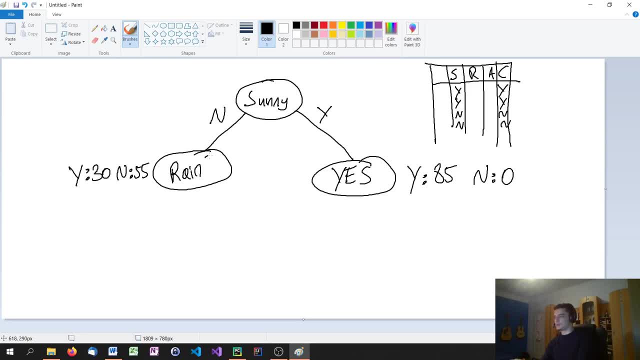 can ask the next, the next question, So I could say: is it rainy or not, Does it rain or not? And then I could split it up again, So I would get again yes and not And all the data rows that have a no in sunny. 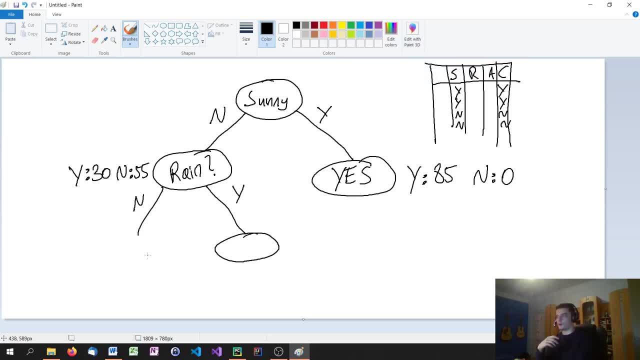 and a yes in rain end up being here, And all which have a no in sunny and no in rain end up being here. And then again I look at the data and I say, okay, if it's not sunny and raining, he has I don't know. uh, 40 nos and zero yeses. So here I. 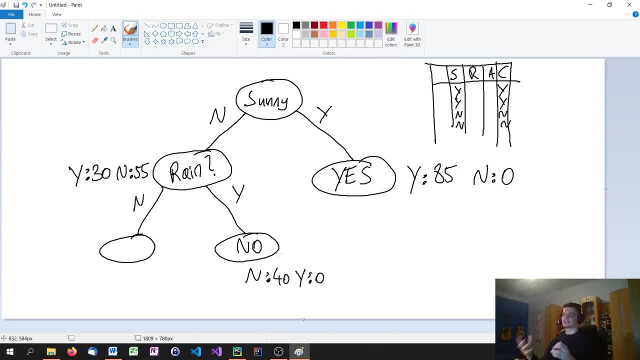 could end and say he's not going, Okay, But if it's not sunny and not raining, I can ask if is he going alone, and then split the tree up, uh, even more. So in the end, I would end up with a model that is somewhat trained. So this is what the algorithm then does: It takes the data and optimizes the decision tree, But of course, we have a random factor here, because which question or which feature do we start with? I can start with sunny, Uh, I can start with rain, And of course, uh, the tree varies, uh, enormously, because if I start with rainy, not every time when it rains, uh, is he not going? So so I could check for rain, get a yes. 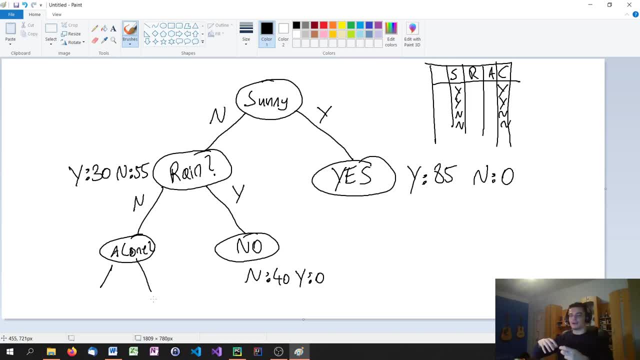 And then I would have to check for sunny. Uh, and even if I get a no in rain, I would have to check for sunny, Whereas if I start checking sunny- checking for sunny, sorry- I end up with a yes immediately. So it's not, um, it's not the same uh, which feature you start with, So it makes a difference. That's what I'm saying. So, uh, this is a random tree and you can have multiple trees with different outcomes or different efficiency, basically, But this is how a basic tree is trained. 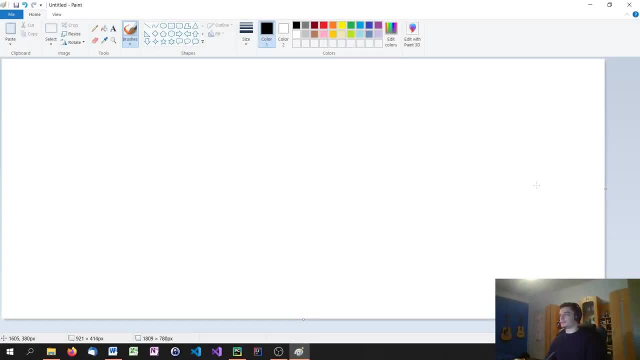 And now this is where random forest classification comes into play, because a decision tree might be kind of random because of the order of the features. So if I have a data set with 50 or a hundred features, the order of features chosen is uh very important and it might lead to uh huge differences in the output. So one decision tree might give me a yes, Another one might give me a no, just because uh the order of the features was picked differently. 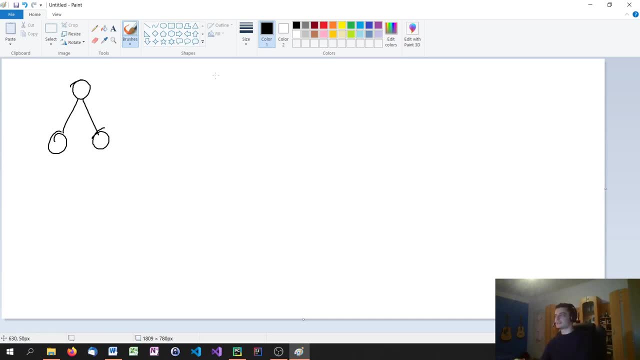 So what I can do is I can start with a no. So what I could do and what I do with a random forest classification is I create multiple decision trees- not only one, but maybe 50 or a hundred or 200 decision trees- And I train all of them on the same data. So this is our data And I feed this data into all these different decision trees in the forest. So a forest is made up of multiple trees And I have all these decision trees trained on the same data, And what I do in the end is I get a new task. 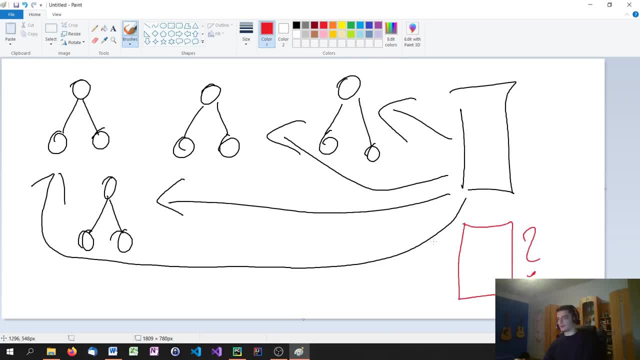 So this is the test example and I want to know what the answer would be. So I feed the test example into all of these, into each of these decision trees, and they will all give me an output. So this one might say, yes, he's going out. This one also says yes, he's going out. This one also says yes, but this one says no. So of course, the collective result of the forest would be yes. So I have three against one, It would be yes. And of course, if I have three against one, it would be yes. 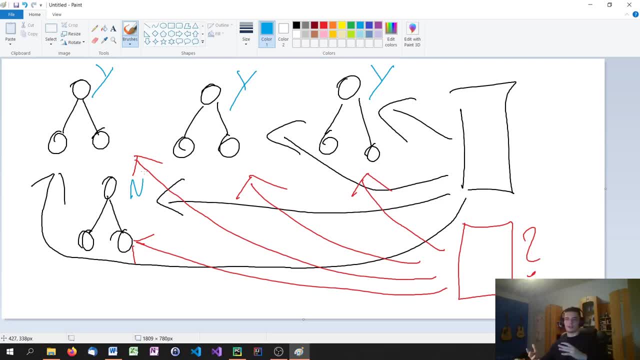 50 trees- it would be something like 44 against 6, for example, and I get a yes, or sometimes it may be not that clear, but basically I train multiple trees to have different opinions more or less on the same issue, and the advantage of that is, of course, that the I minimize the risk of a. 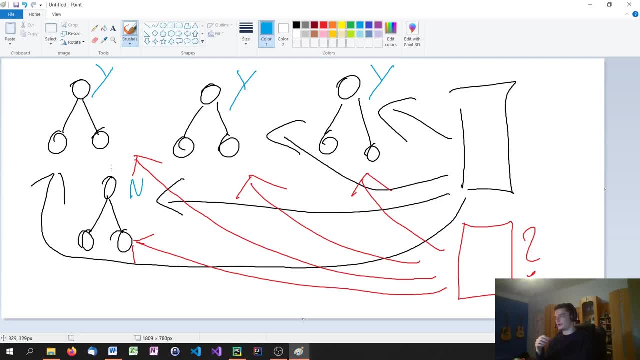 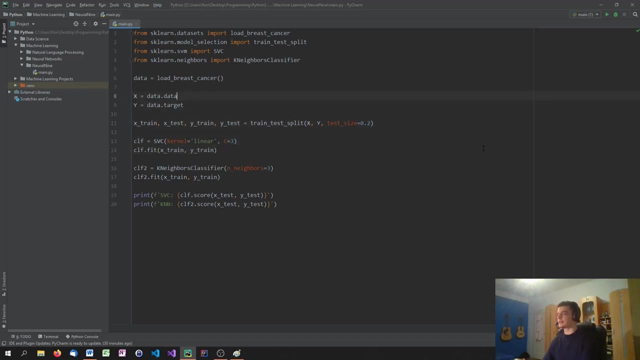 misclassification, because if, for some reason, I end up with only this decision tree here, I get a no, even though most other decision trees would end up with a yes. so a random forest basically uses a democratic system of classification with multiple decision trees. so let's look at the implementation in python once again, and this is the code from the last. 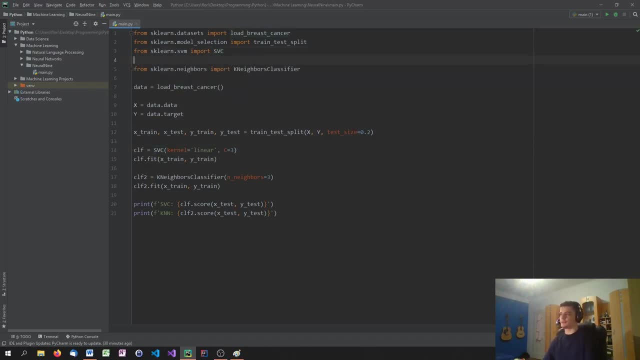 video and we're not going to add too much new stuff. we're just going to use two more classifiers. so the focus of these initial episodes is to get to know as many algorithms and classifications and regressions as possible, and later on we're getting into some deeper topics, but for now we're just going to test different models to 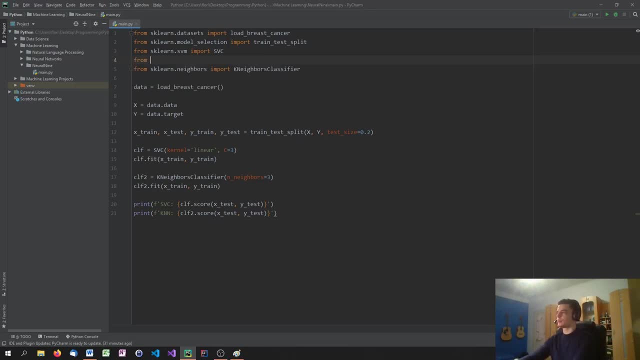 explain how they work and for this reason, we're going to just import from sklearntree- I think, yes, from sklearntree- import decision. tree classifier. we can also have a regressor if we want to do regression, of course, and we're going to import from sklearn. dot wasn't forest, what was it? 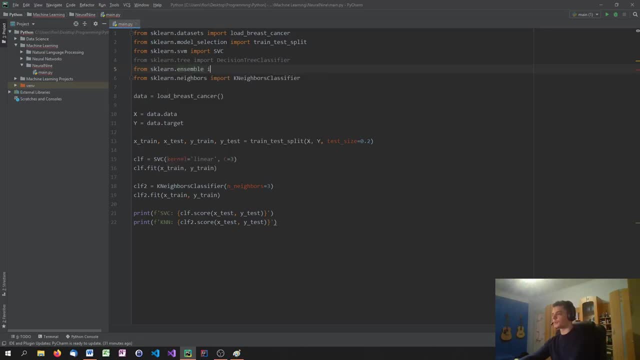 dot ensemble, I think. import random forest classifier- yes, or also regressor, if you want so- from sklearntree. import decision tree classifier from sklearn dot ensemble. import our random forest classifier. and what we're going to do now is we're going to define a third classifier, equals. 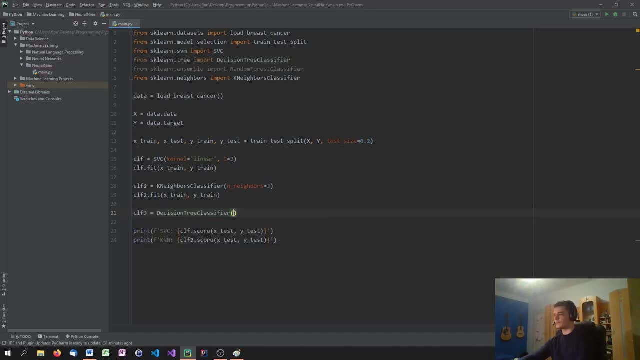 you decision tree classifier and we're going to fit that classifier on the training data- X train and Y train- and then we're also going to define a fourth classifier, which is the random forest classifier. let's look at the parameters here, yeah, and then we can also define how many samples we want to offer, how deep it. 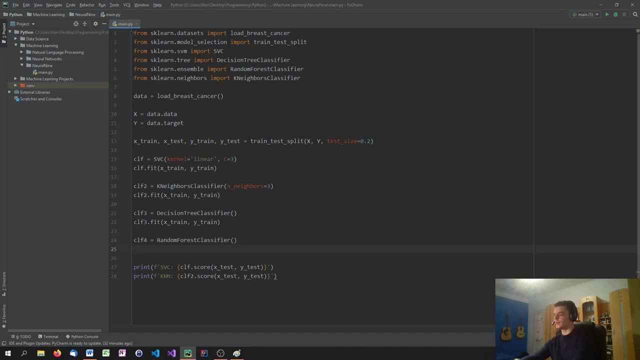 should go and so on. we're going to leave the default value. so classifier for dot fit, X train and Y train, and we can now print and compare the results. so we're going to say this is the decision tree classifier, DTC and the random forest classifier, and here we say cof3 and cof4.score. so let's see how the models perform. 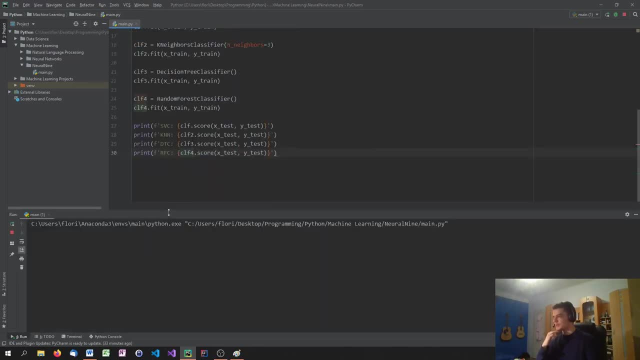 maybe they outperform the support vector machine. i don't think so, to be honest, but let's check out. um, so in this case, the random forest classification is as good as the k neighbors classification, and they're both better than the support vector machine and the decision tree. 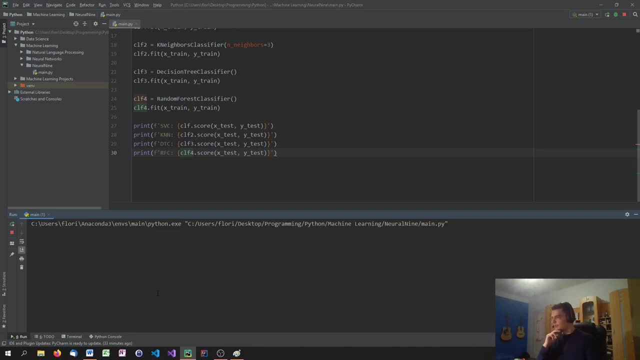 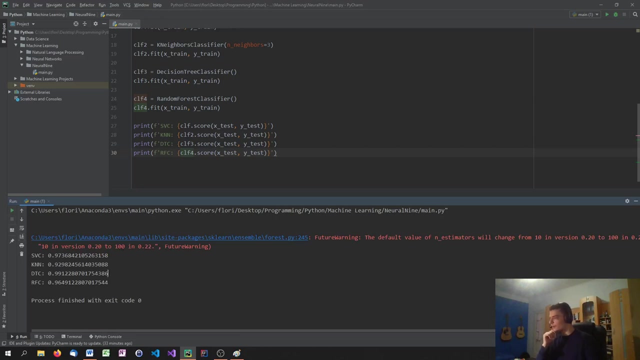 classifier. let's see what happens if i run this again. we end up with nothing, takes a while, is it laggy or something? let's run this again. oh, there we go. uh, in this case, the support vector machine was had a 97 percent uh accuracy. the decision tree classifier had 99, which is 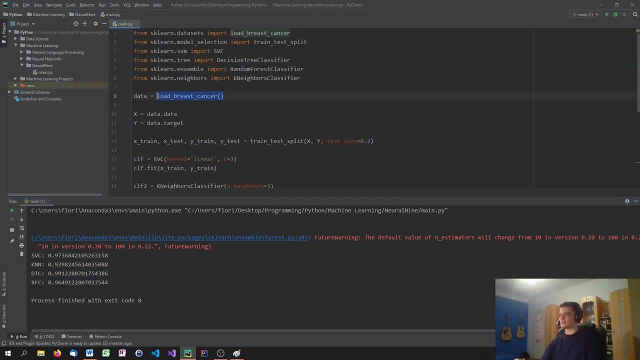 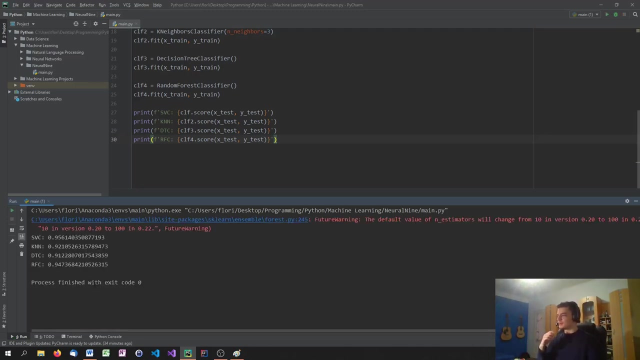 very accurate. if you think about, uh, breast cancer data, this is: this is crazily accurate. so, uh, and also the random forest classification has 96.. but of course we had one decision tree that was 99, 99 accurate, sorry, so it's also a little. 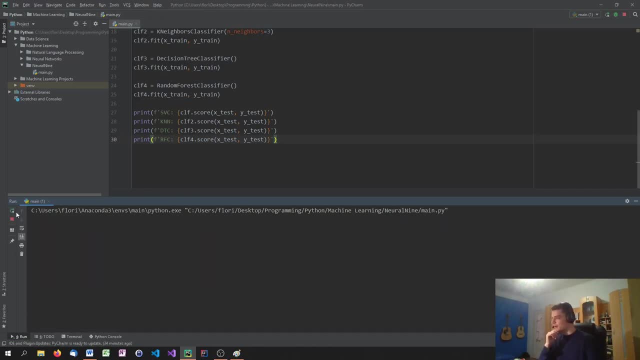 bit of a random factor in there, but you can see that on average we have the same performance. so the decision tree maybe is not that accurate, except for this one case where it had 99 uh. random forest, though, is pretty accurate most of the time, so this should be a good algorithm for.